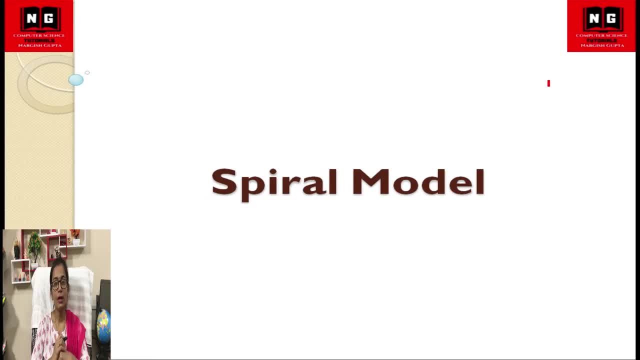 software means the basic focus of the spiral model is risk analysis of the projects. so basically, this spiral model is used in complex projects because the main point of this model is risk analysis. so in complex projects, risk analysis is very important, so usually people like to prefer this model. so let's start with what is spiral model? 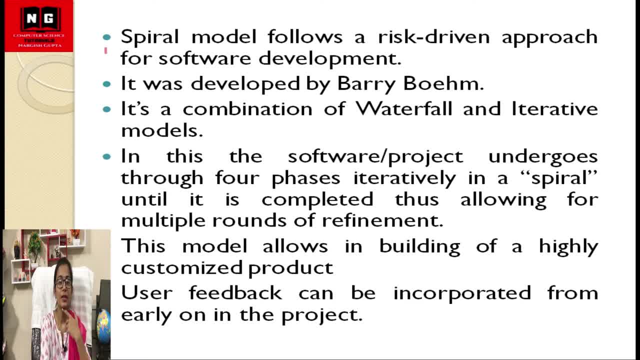 so, coming to the first point, what it says is that spiral model follows a risk-driven approach. main point of our spiral model is that it follows a risk-driven approach of software development. the steps are same almost, but their nomenclature changes means their naming changes and the way of following those same steps. 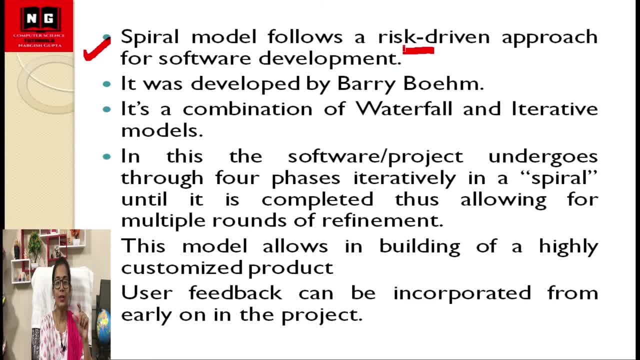 changes. so what we saw in this main point is that this is a risk-driven software development process. what is the next point? it was developed by barry boehm. barry boehm developed it. the next point: it's a combination of waterfall and iterative model. 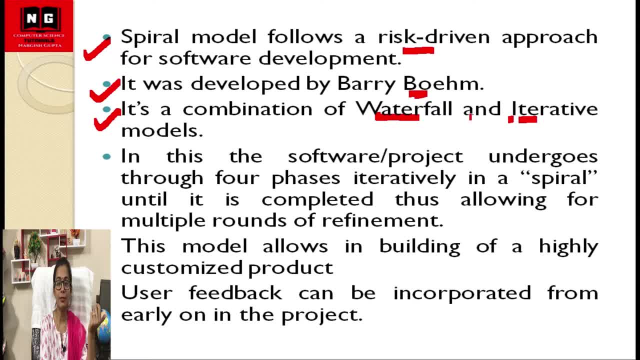 these are the two models which we have already studied before. so these are the this spiral model, basically based on this two models, that is, waterfall model and the iterative model. now, coming to the next point, what does it say in this? the software project undergoes through four phases iteratively in a spiral until it is completed, thus allowing for multiple rounds of. 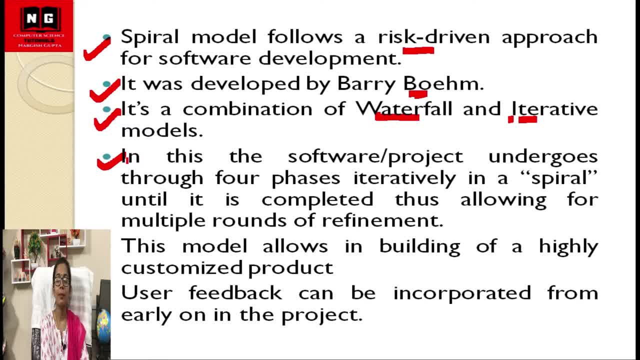 refinement the software project undergoes through four phases iteratively in a spiral until it is completed, thus allowing for multiple rounds of refinement. means spiral model. means in last spiral model there are four phases which continue to work through the spiral. how can you imagine a spiral? you see a montan coil. 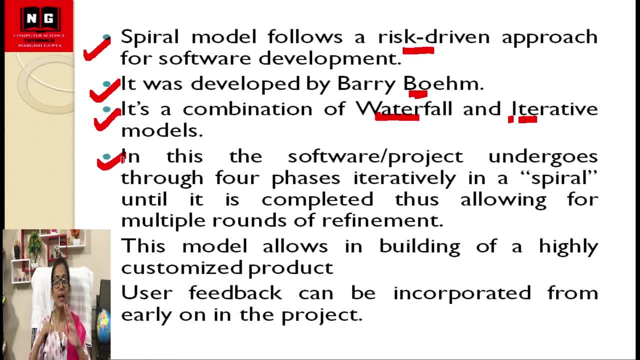 it is spiralling in this way. so basically, we divide the project into four quadrants and continue to work on a single spiral and each of our projects are, revise occurs and every project is in the aspect of one project and under construction. that is the model. our companies do not consider rundown project optionesto and we. i came to know that that is great and if you think about it, 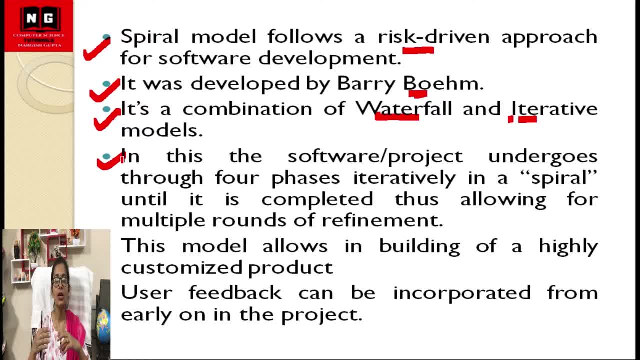 spiral pe humara project aur refine hota jaata hai aur evolute hota jaata hai. yeh wali baat, iska evolution pe evolution hum karte jaa rahe hota hai, har ek spiral pe. now coming to the next point, is: this model allows in building of a high, highly customized project. 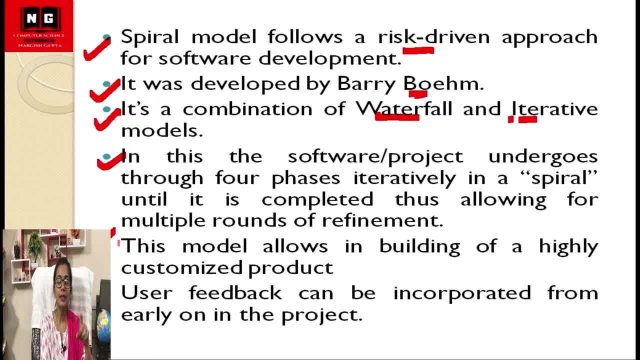 customized project. kyun jaate hai kyuki har ek step pe bhi hum aage, jab iske phases dekhi inge. toh aapko yeh cheez zyada clear ho jayegi kyuki har ek spiral me hum customer se review. 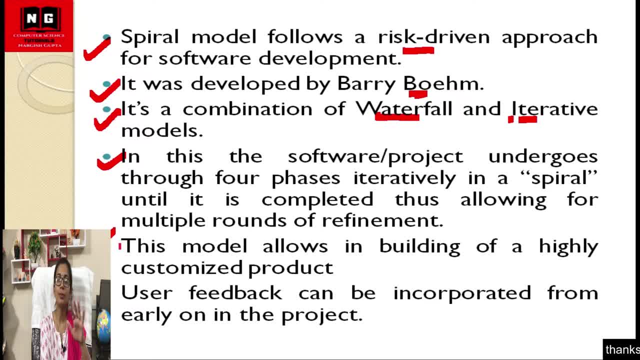 karwa rahe hai, customer se evaluation karwa rahe hai, toh isme proper customized projects achche se ban jaate hai. now the last point is: user feedback can be incorporated from early on in the project. toh user ke feedback kya hai? hum from starting phase hum include. 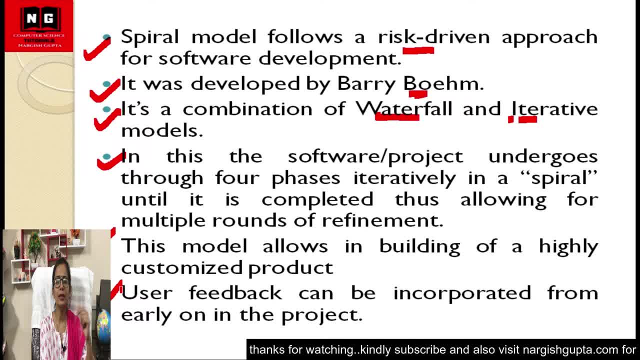 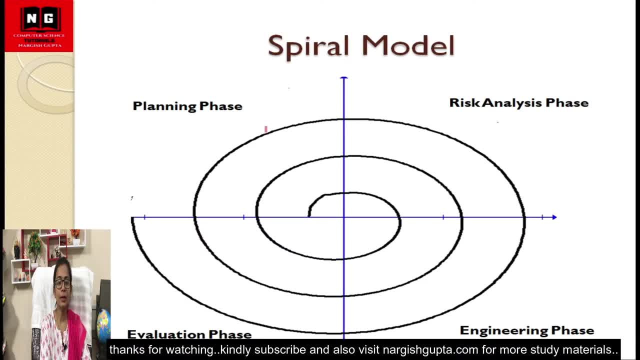 kar rahe hain. toh thus it helps in building a better quality and less error prone software. ok, let's come to the phases first. so yeh aap, yaha pe hum luk, jo dekh rahe hai, kya hai yeh four quadrants, hai yeh humara first quadrant, aagaya yeh second quadrant, yeh third quadrant. 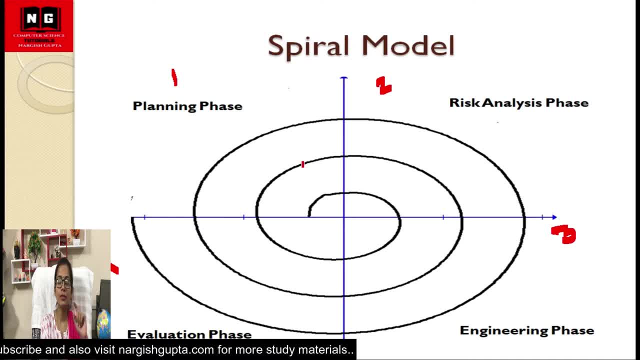 and this is a fourth quadrant. toh first quadrant, kya deal kar rahe hai? planning phase se planning phase, hum yaha pe SDLC ke phases ko hum yaha pe include karein, toh yaha pe humara. basically, requirement gathering or analysis is required, so we have to include the phases of SDLC here. 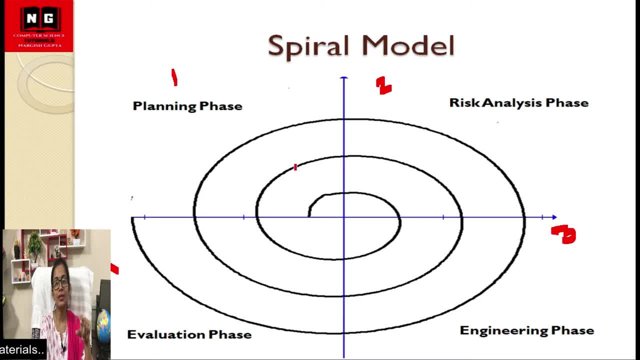 and if you are a touch, this will help you getting this bit work out here, because whether CM and Process analysis, whala tho VC raha ai planning basis ki vau lah brother. so I wasn't much ensuring that kya is OCM? accha asine hain par problema you fund transfer, so we 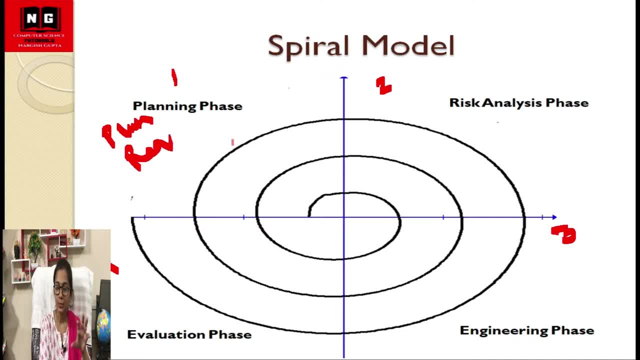 have to. MR tohיי ke. yeh, right, so we have done that. Q an S T I th e planning. we have done an analysis. wala thoda aissa par art has gone. that planning like this, which we have done, that diligants par item almost 3 months have to, you can have worked in process. we have worked in a separate. 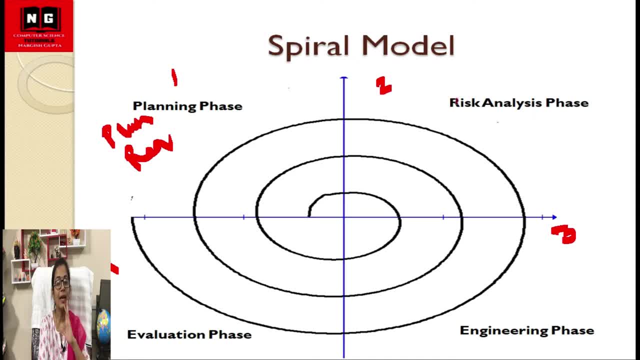 project. project planning plus requires analysis. waya pul-da part aai planning phase ke under hum project karna. shuru karenge toh risk analysis phase pe kya aate hai yahan pe aate hai. risk analysis phase pe jen requirements mein work karne jaa rahe. hota hai toh unke pehle risk ko analyze. 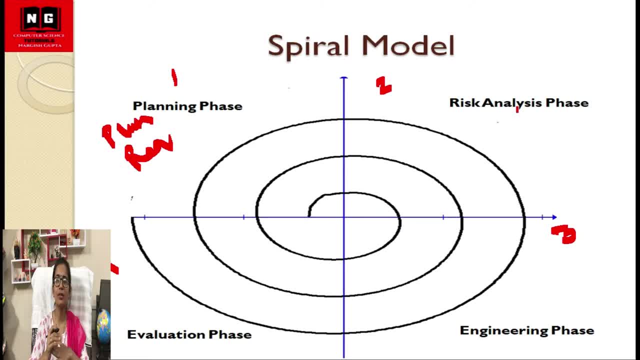 karte hai. matlab suppose, if we have any project in which there are ten requirements, toh ten requirements mein. se suppose we are working on three requirements in the first spiral, aur un tino requirements ki hum sabse pehle risk analysis, karenge risk analysis basically. 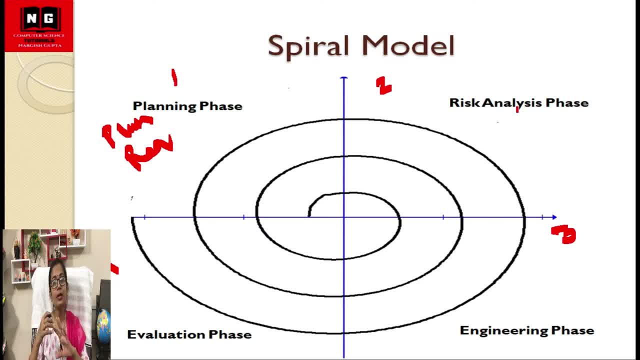 kya ki agar hum usse develop karenge, toh aisa toh nahi hai, ki kahin pe hume bahut issues aane ke chances hai. yaa, kya complexity hai. toh uski proper complexity ko analyze karenge. 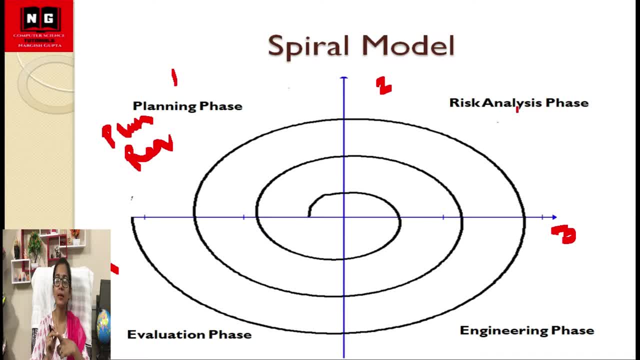 toh is yahan pe risk analysis, hum kis tarike se karenge hum risk analysis, yahan pe prototype bana ke karenge kyunki hum kuch working, karenge kuch coding, karenge tabi hume uske exact analysis. 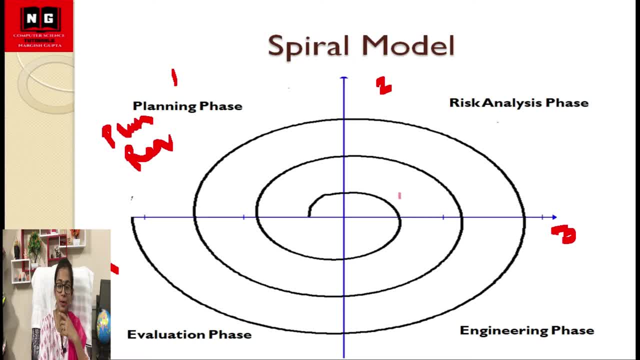 hai exactly risk ka idea. lahega toh hum har ek spiral mein yahan pe kya hota hai ek prototype. banta jata hai jasain yahan pe kya banyan jayega P1, P2. har ek spiral pe ek ek prototype. 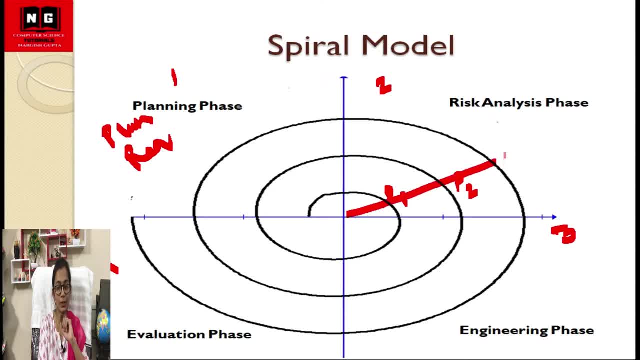 humara yahan se evolute hota rehta hai. is tarike se toh yahan pe risk analysis humne kara risk analysis kara prototype. ban gaya prototype humara jab finally ban gaya usse. So we came to the next phase here, in the engineering phase. so what did we do now? the prototype was developed. now, which things will it deal with? 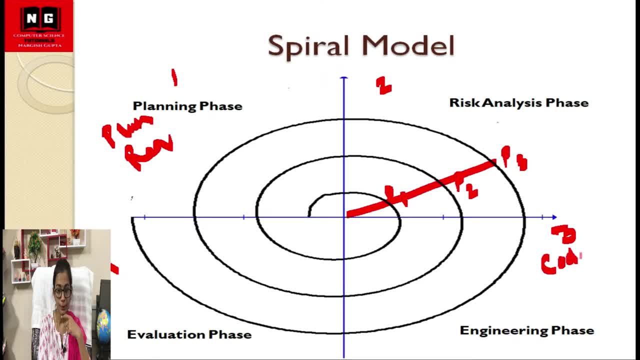 This is our coding, testing and deployment. So this coding, testing and deployment, who will deal with these three things? our engineering phase: In this phase we will do the actual coding of the prototype, that is, the actual development of it in this phase, plus its testing and deployment. 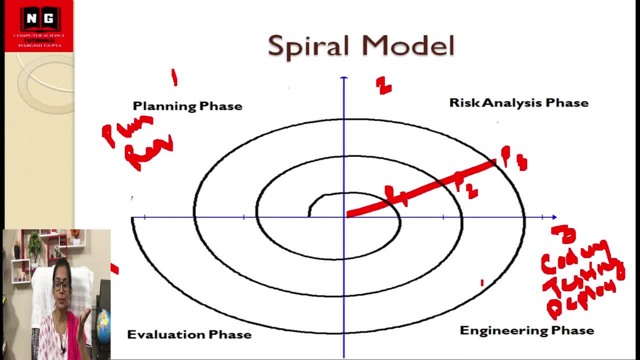 Deployment means we handover that client to the project. So our next phase is called evaluation phase. What will it do? Here comes the customer evaluation, here comes our customer focus. So here we will do evaluation from the customer, for whom? for our project that we have made. 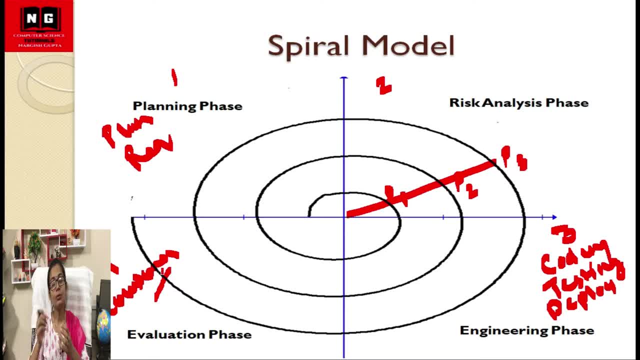 And what can be the add-ons in it, or if anything is missing, then how to overcome it, if there are any issues, and we will properly analyze the risk. So here we will do evaluation from the customer And then from here, what will we do again, 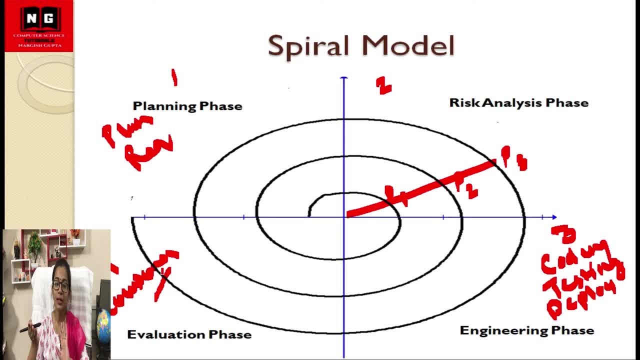 We will decide whether we have to go to the next planning phase or not. If we have to go to the next planning phase, then again we will come to our second spiral here. then we will move here. After coming here then, some of the requirements, the feedback we had at the back, plus if there are any bugs left here that we have not dealt with. 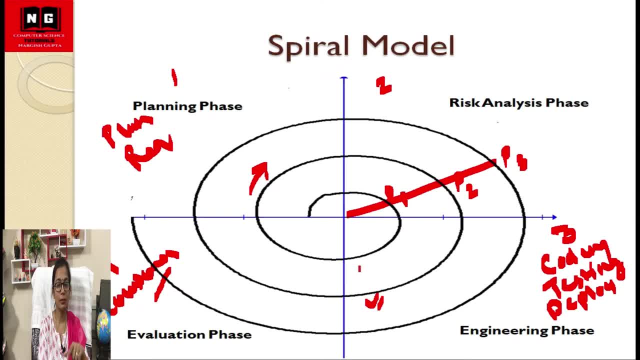 If there are any bugs of this phase and we have not resolved them, not finished them. So what will we do? We will take it here and go. That too will come in our risk analysis phase in the way of a requirement. Again, we will develop the prototype, our P2.. 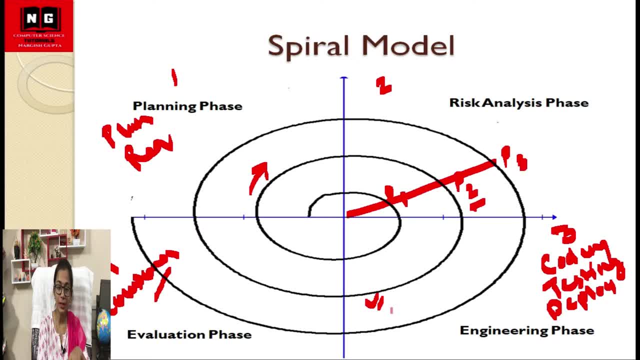 P2 will be developed According to that, again by coding in the same way. a spiral will go on and on until all our requirements are completed, And in every phase our project is getting more refined and evolving. This is our basic working of spiral model. 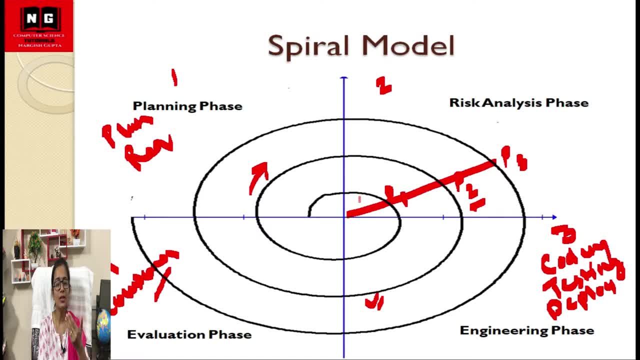 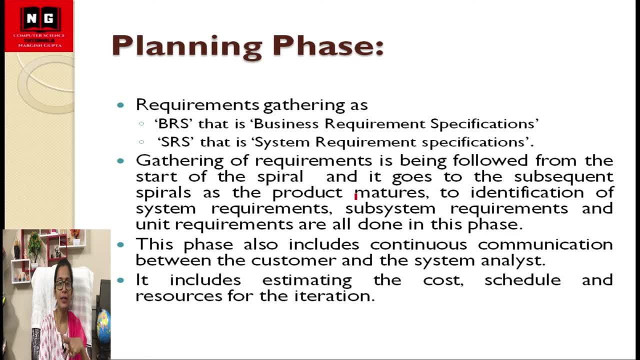 Let's see the theoretical points related to these all four phases. So what is our planning phase dealing here? Requirement gathering, as we have said, is dealing with requirement gathering. These are SRS and BRS. According to them, we decide our things here. 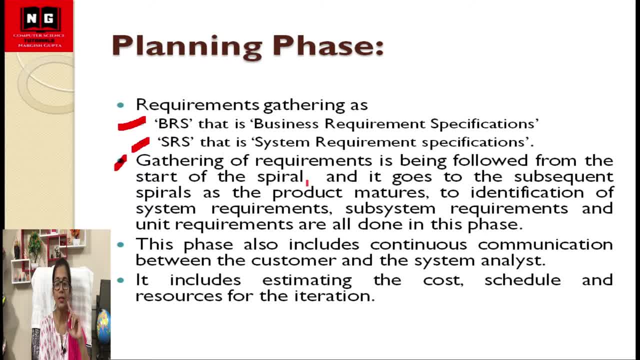 Then what is the next point coming? Gathering of requirement is being followed, Meaning how do we do gathering? Followed from the start of the spiral and it goes to the subsequent spiral as the product matures, to identification of the system requirement, Sub system requirements and unit requirements are all done in this phase. 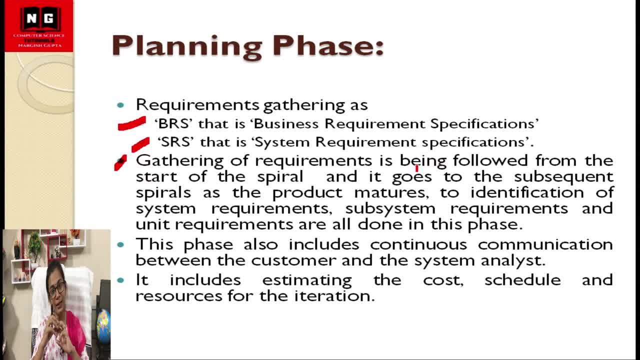 In short, what is he saying here? We do requirement analysis in this in the starting. Then what happens in every phase? We have analyzed some requirements once. Then what is being done every time, Meaning the feedback of the previous phase is being done. 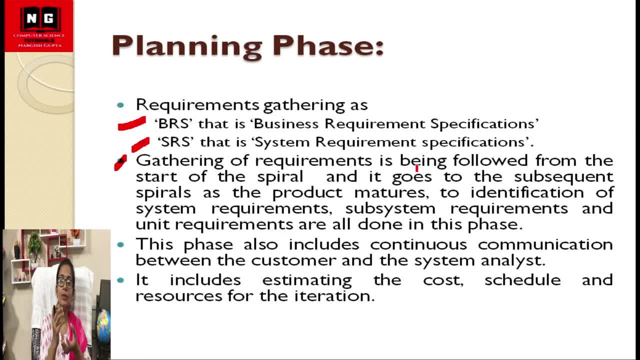 Plus, now the first requirement gathering that we did, we did it on the basis of a particular project. Then, as it is getting matured, then we do requirement analysis according to the system, Sub system, according unit system, according Meaning. first we did requirement gathering of a unit. 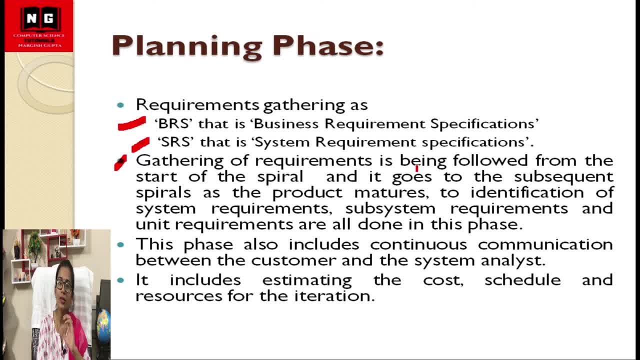 Then we increased its number of modules, Then we went to the entire modules. So what is he saying in that way? He is saying that we evolve our SRS in a new way on every spiral. Now the next point says this phase also includes continuous communication between the customer and the system analyst. 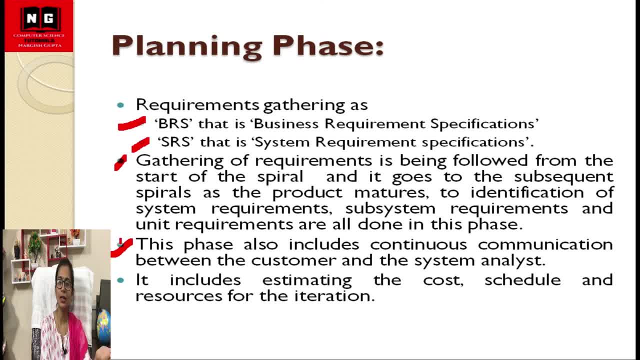 Because requirement gathering is happening, then requirement gathering can't happen without the communication of the customer, So that's the same that they must be communicating Now. then last point is it includes estimating the cost, schedule, Schedule and resource of the iteration. 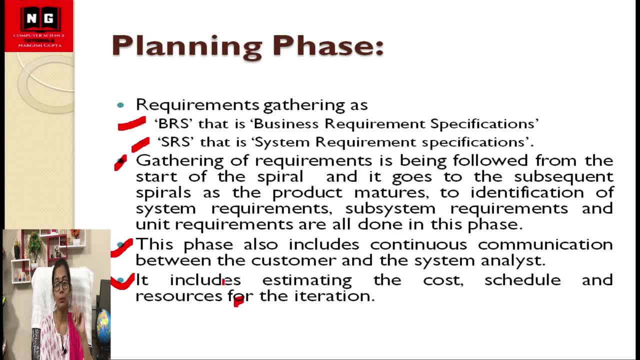 Resource for the iteration In this planning. in our planning phase of SDLC we used to do this only. We used to finalize the resource. So in this also we will finalize Requirement plus resource, schedule cost. Everything has been decided. 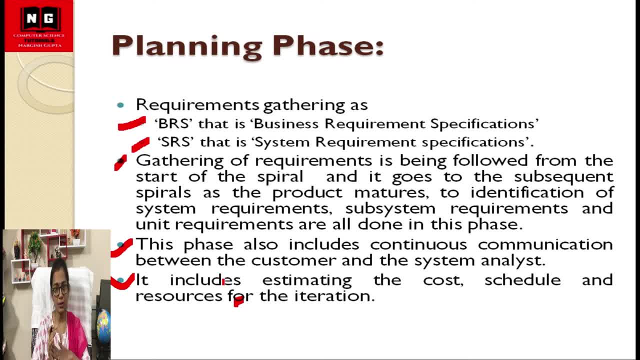 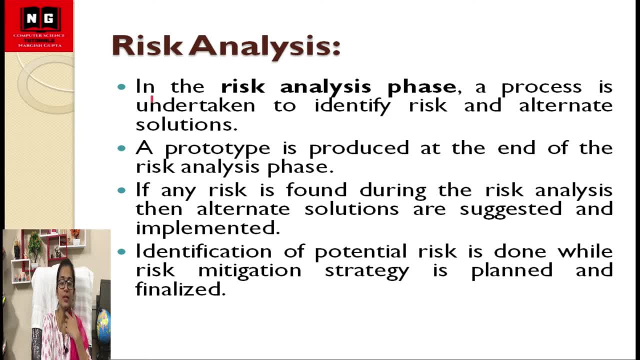 Now, after deciding what will be our next phase- Risk analysis phase- Let's see risk analysis phase. So, coming to the risk analysis phase, In the risk analysis phase, a process is undertaken to identify risk and alternate solutions Means if there is any risk in a particular project. 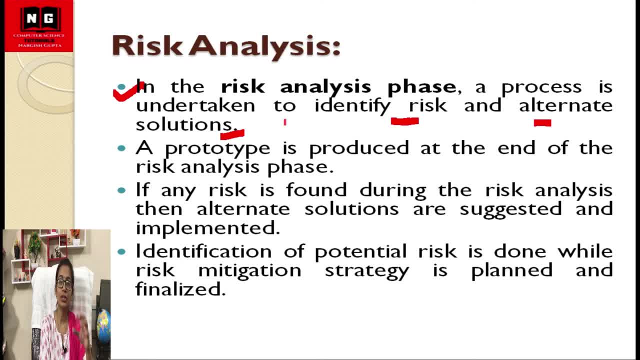 We get to know. So we will create an alternate solution of it Through which we can overcome it. So a prototype is produced at the end of the risk analysis phase. If any risk is found During the risk analysis, Then the alternate solutions are suggested and implemented. 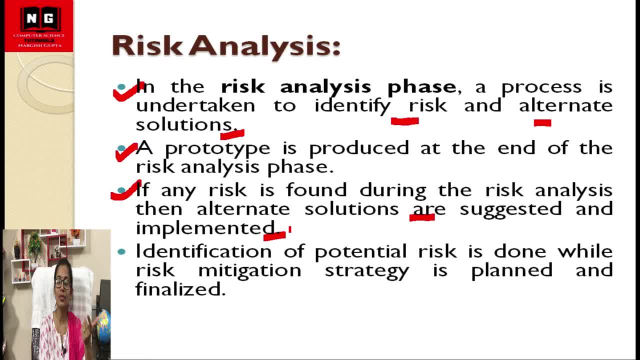 Means. if we are suggesting Thus, we will implement those in that Developing a prototype also. Last point is: identification of potential risk is done While risk mitigation strategy is planned and finalized, Means we see that if this risk is very big And we are not able to solve it here, 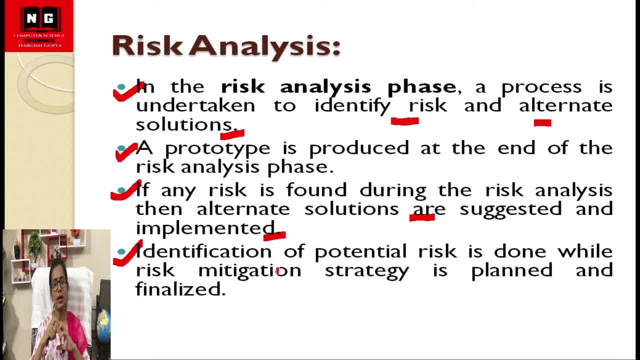 We are not able to solve it. Some such risks come Or some such issues come. There are chances in the project That we are not even confirmation, And there are chances too. So we think that, okay, Let's do development If some issue. 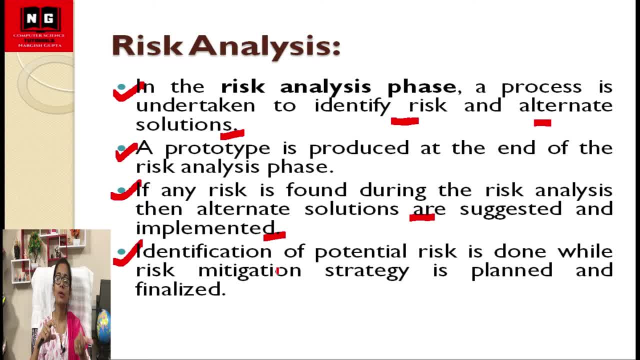 Which we are feeling that it can come That we will continue it in the next spiral, after further evaluation On that analysis in the next spiral We will find its solution. So what do we do? We mitigate it Means for a spiral once. 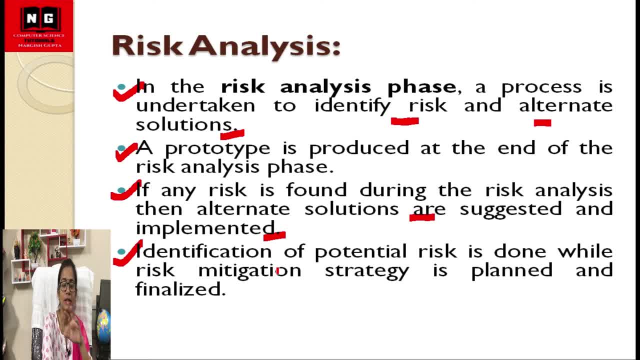 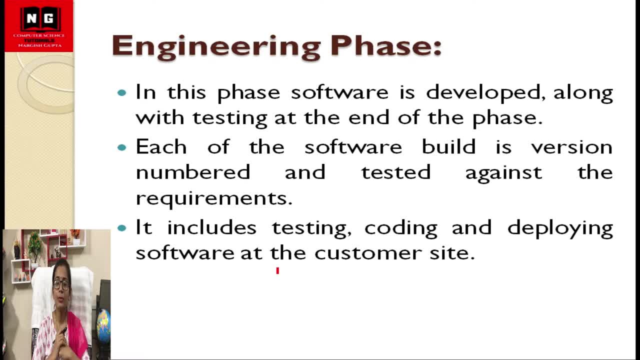 Then we will postpone it. So that's all for the risk analysis phase. Now coming to the next phase, That is the engineering phase. What is our engineering phase saying here? That in this phase There were three main things in it: Our coding, testing and deployment. 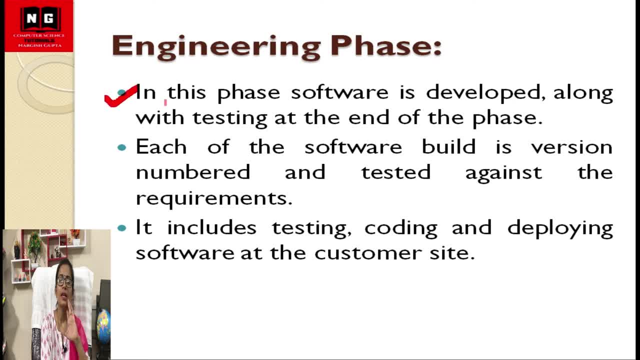 Thus, it will deal with these three things. So what is it saying in this? That in this phase, software is developed along with testing. At the end of the phase Developed, the software Testing is also done. Each of the software built is version numbered. 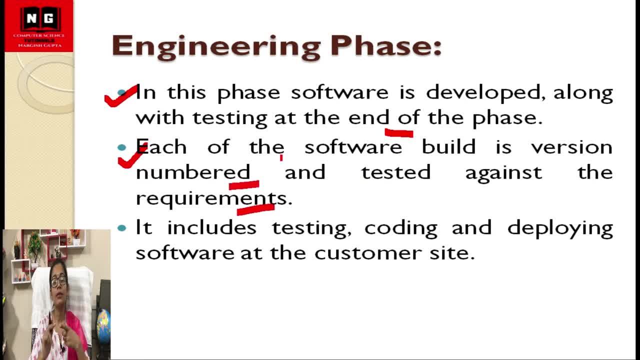 And tested against the requirement. What is version numbered Means? every time a particular software is being made, A software is coming out in every spiral. A version of software is coming out in every spiral. So every time, whatever our software is made and completes in a spiral, 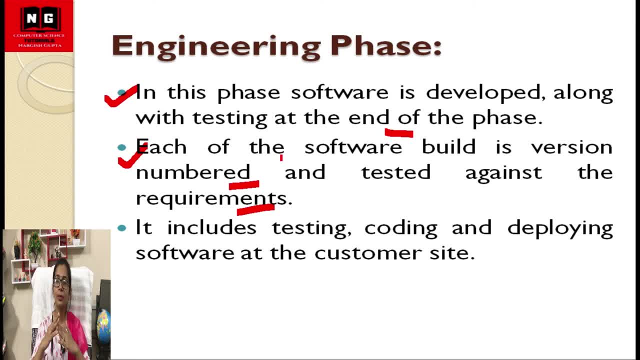 We give it a version. Suppose our first version is 1. So next is 1.1, 1.2.. In this way we numberize the version And, according to testing Whatever requirements we had gathered in the planning phase. 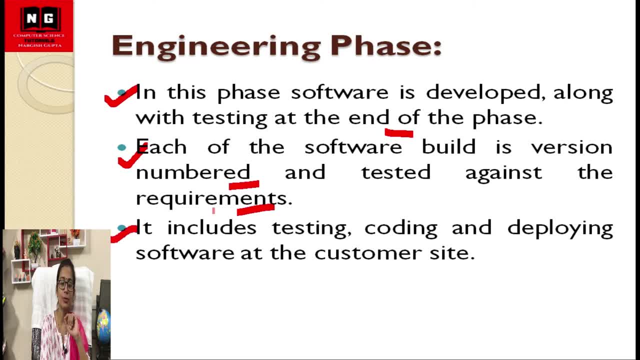 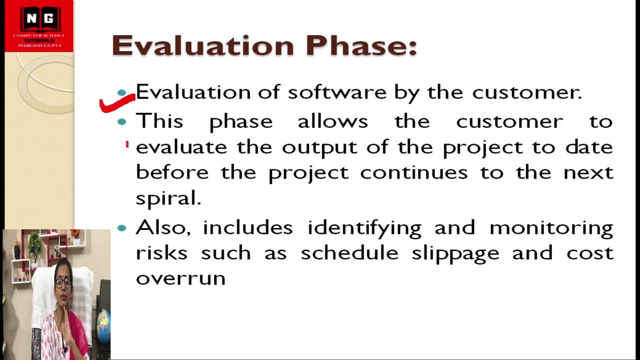 Against that we complete the testing. Now coming to this point that It includes testing, coding and deploying software at the customer side. That's it Coming to the next phase, That is, the evaluation phase. What does it say? Evaluation of the software. 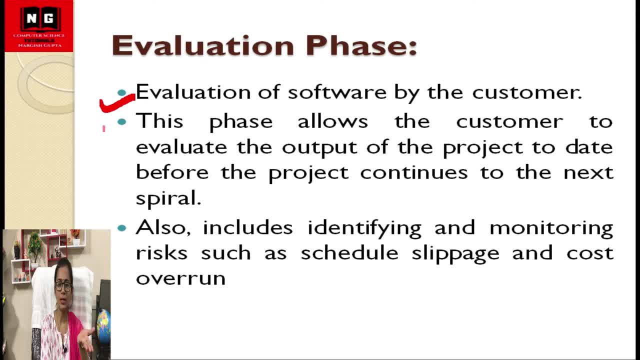 Of software by the customer. Here software is evaluated through the customer In this phase. Allows the customer to evaluate the output of the project to date Before the project continues to the next spiral, Means before we go to the next spiral. Proper evaluation is done from the customer side. 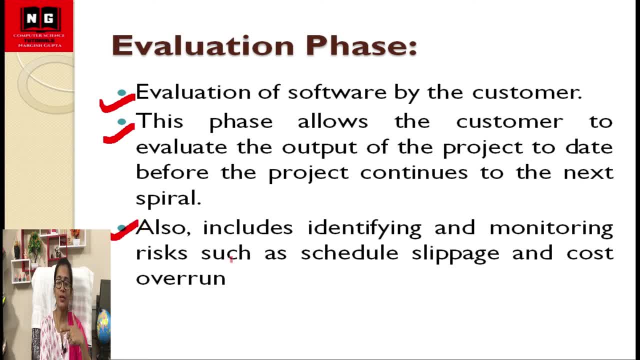 Also includes identifying and monitoring risks, Such as Schedule slippage, Cost overrun Means. it is not like this One. we are seeing the risk related to the project there. One: we are seeing the risk related to the software development. Is it not that our schedule is slipping? 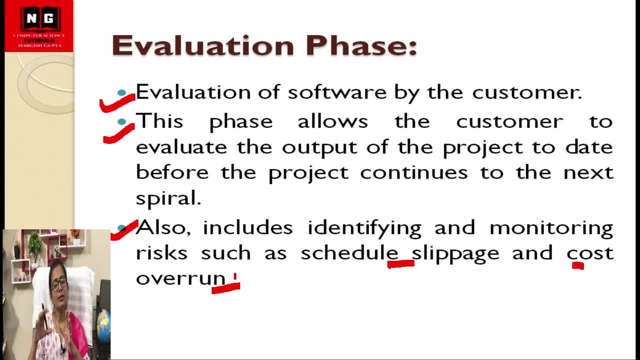 Cost overrun is happening. So, after executing all these types of evaluation here We start the next spiral, So that Whatever is the feedback of our evaluation phase Or output That is used as an input in our planning phase. So that's all for the phases of the what we say spiral model. 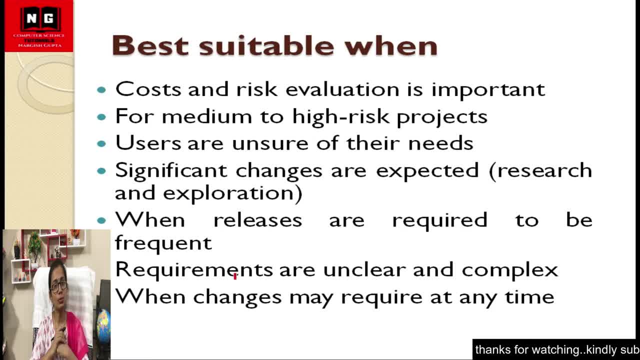 Now come to the next point. That is best suitable when Means what type of projects will be suitable for our spiral model. So we have come to the first point. What is it saying in this? Cost and risk evaluation is important. In which projects the evaluation of risk and cost is more important? 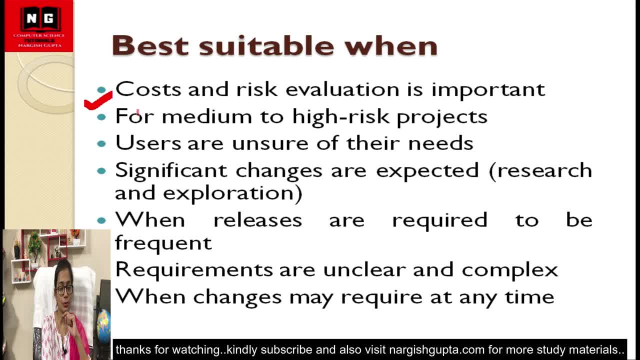 In that type of project. In that type of project, We will use it. Next point is for medium to high risk projects. We will use it. in medium to high risk projects, Users are unsure of their needs, Means the user is still deciding what the requirements will be. 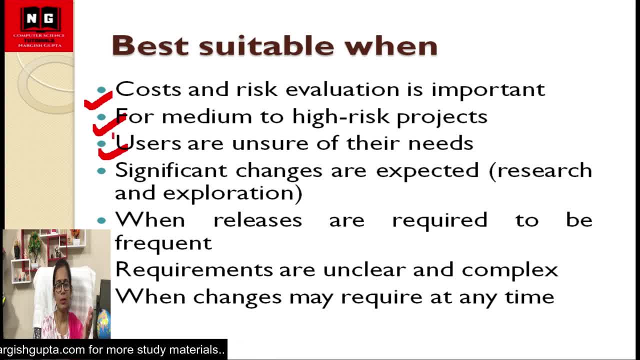 So accordingly, we will evaluate it slowly And slowly we will take in the requirements. So we will work on whatever has come And move forward. So in that type of projects we will basically use it. Then significant changes are expected, Expected Means why 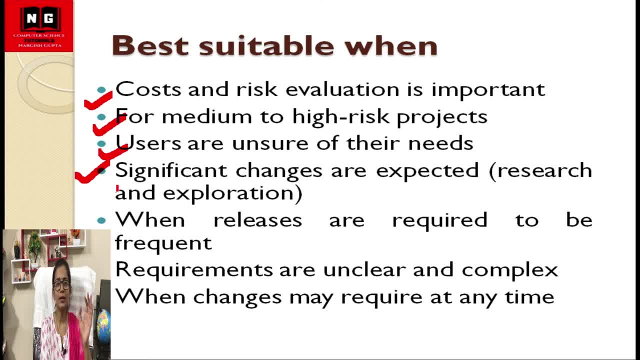 Because there are chances on every spiral To accept different types of changes. That is why it is good for a project In which there are chances of many changes. Like we have given an example in this, Like research or exploration Means, we are trying to explore something. 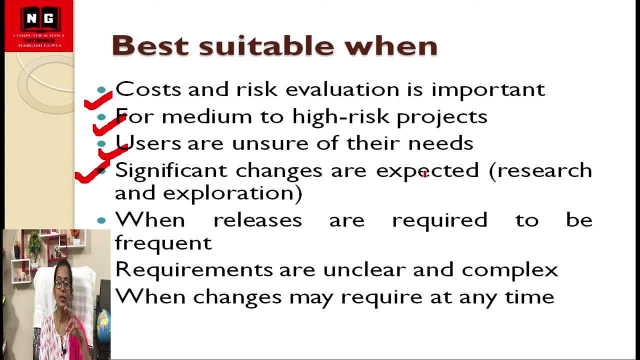 That if we will make this project, Then how will it be made? What will happen? So in that type of project we can use spiral model. Now next point: what does it say When releases are required to be frequent? Requirements are unclear and complex. 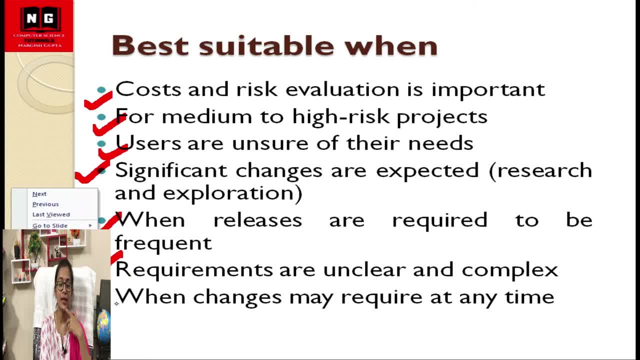 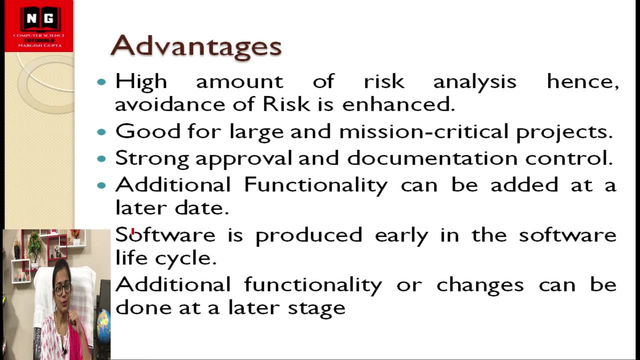 When changes may require, at any time, So whenever changes are required. According to that, in these types of projects, We can use spiral model. Now coming to the advantage of spiral model. So what does it say? High amount of risk analysis, Hence avoidance of risk, is enhanced. 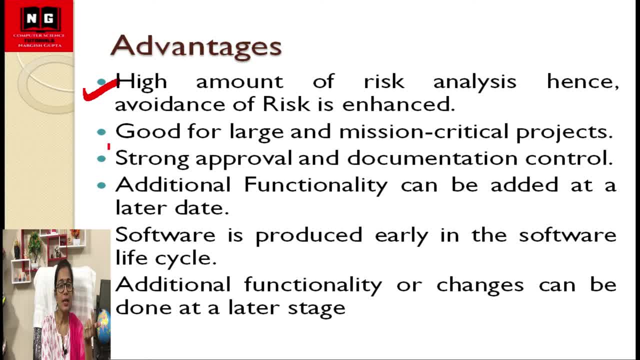 So what advantage we have got When it is focusing more on risk analysis. Hence, in our project, we are able to avoid risk From starting of the project itself. Now coming to the next point. That is good for large and mission critical projects. 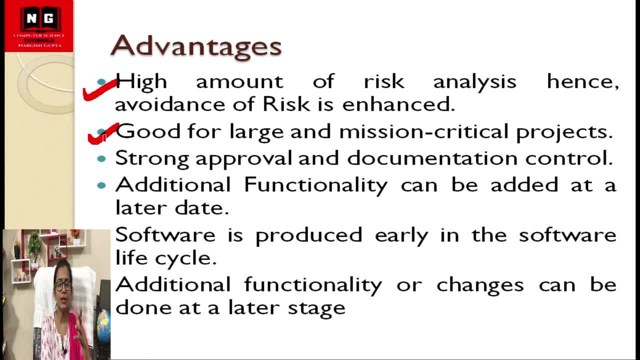 Yes, critical projects, Critical projects, complex projects- For this type of projects, this is very good. Strong approval and documentation control. Proper documentation is going on in this, Because we work on some requirements, Then we develop it completely, Then we work on some requirements. 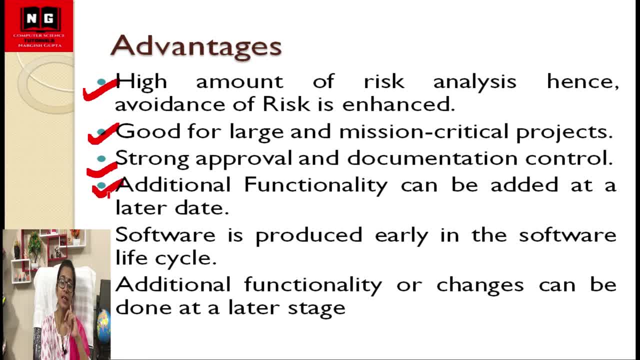 That's why Additional functionality can be added at the later end. If we have to add something, then also we can add it easily Means we can handle change request very well. in this Then software is produced early in the software life cycle. Additional functionality and changes can be done in the later stages. 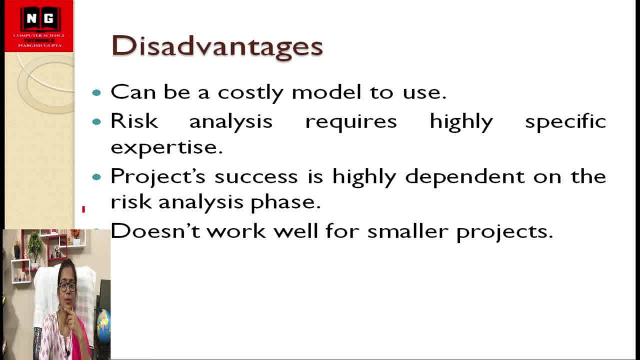 Same point. So now coming to the next point is disadvantages. What are the disadvantages? Can be a costly model to use. Why? Because we are making prototype in this, Then we are developing it, Then prototype, Then prototype will also gain a different cost. 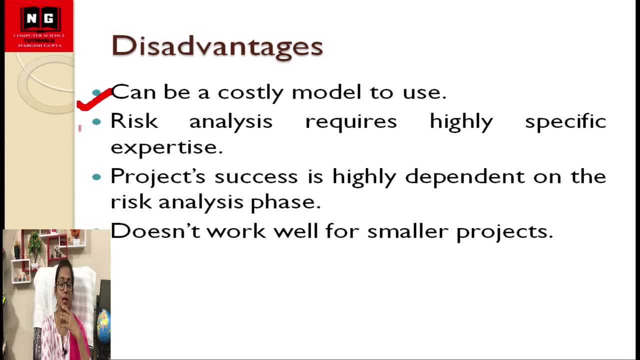 Plus, the cost of development will be there Because of this. Now coming the next point is: Risk analysis requires highly specific expertise. Yes, this is the point. Why are there disadvantages? Because if we are doing risk analysis, Means we should be expert in that area. 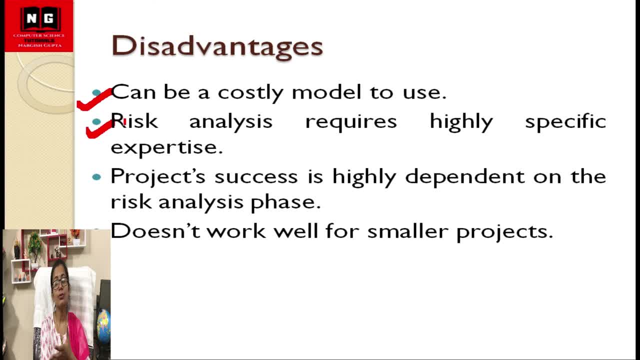 Then only we will be able to analyze the risk of something without developing it, Without going ahead. So means Expertise is very important. So in this highly expertise resources should be there Now. the third point is: Project success is highly dependent on the risk analysis phase.